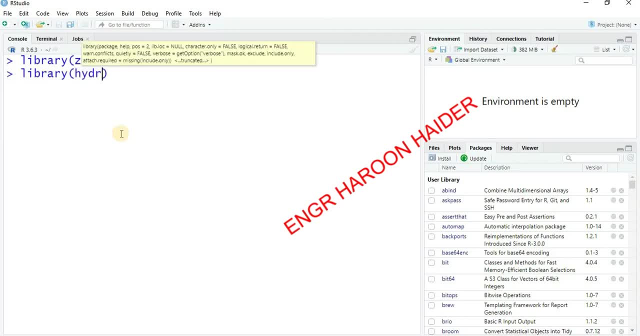 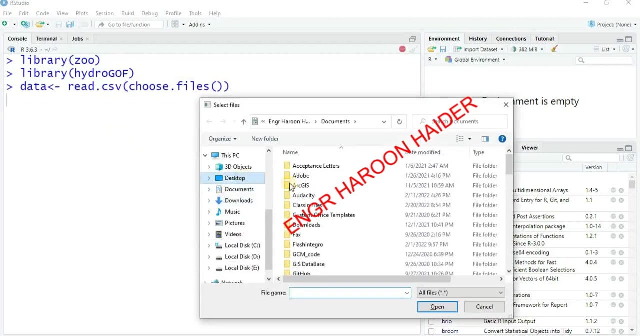 of hydro gof. okay, so, after installing these two libraries, let's upload our data. so, as you, all of all of you know maybe how to add our data, so I'm going to use, as readcsv, same method: choose files and let's choose. I'm going to select the data files for my data, such as a flow dot CSV, as I 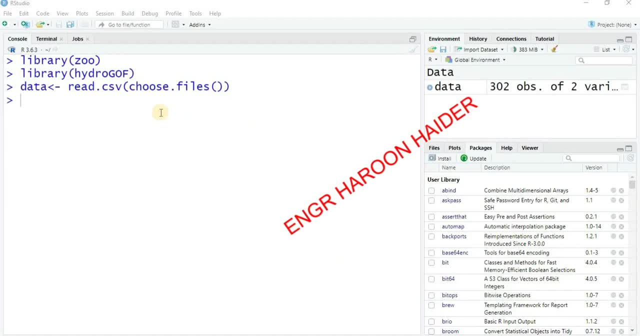 already showed you. okay, so there are two, three hundred and two variables of two, observation of two variables. okay, now let's we have two type of data. one is observed. okay, first get observed data, so as dot, numeric, because we are working with the numerical data, so as of numeric and data, dollar sign and select observed. so 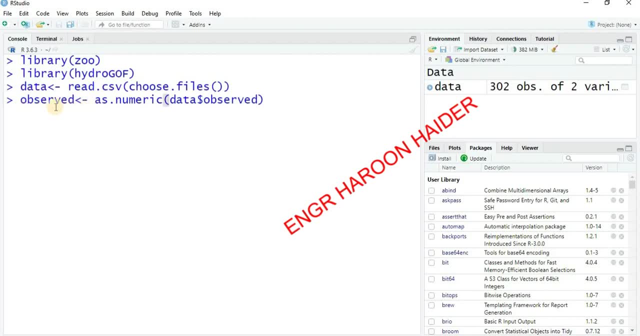 because this observed in this variable. out of that data will be taken. similarly, we are going to use simulated data, so write simulated and in simulated we are. we want to put our data so as numeric same way data, dot, dollar sign simulated. okay, now we have done our all this work. 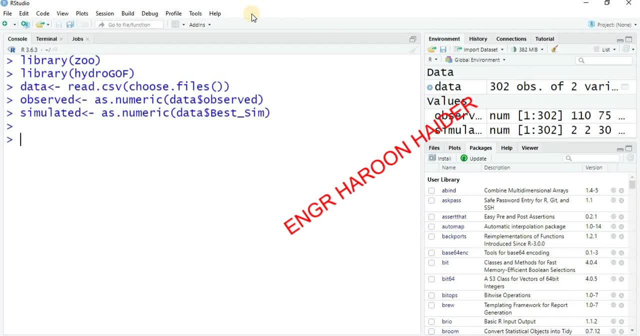 now we need to write our code, a simple one. it is a qf and in qf we need to write simulated, simulated is equal to our simulated data and similarly comma and observed, and in observe we have to write our observed data. okay, I'm just simple, command and 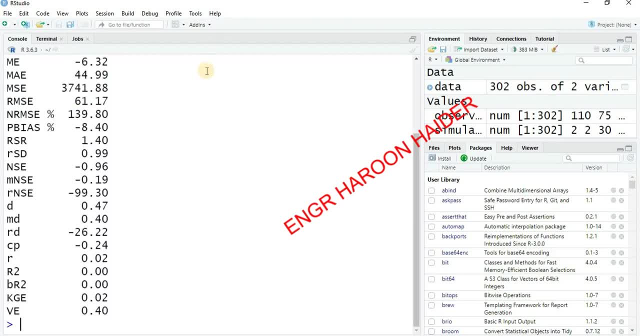 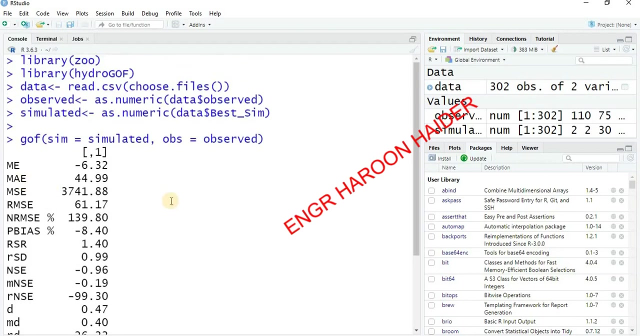 just put enter so you can see all of your possible errors are defined. you can see me. ma e mean error, mean absolute error, standard error, root min, square error and multiple errors. all of these errors are defined, listed, just in a single click. thanks for watching my video. I hope this will help you in your research.